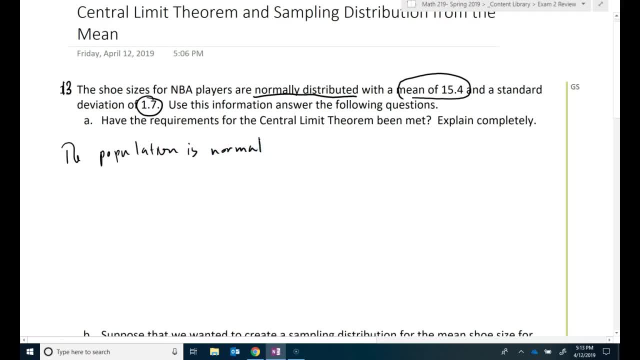 here And I'll explain this to you guys, And what the answer is to this is really important, And it's gonna be important for using the central limit theorem too. So first A asks us: have the requirements for the central limit theorem been met? And explain that completely. Well, there are. 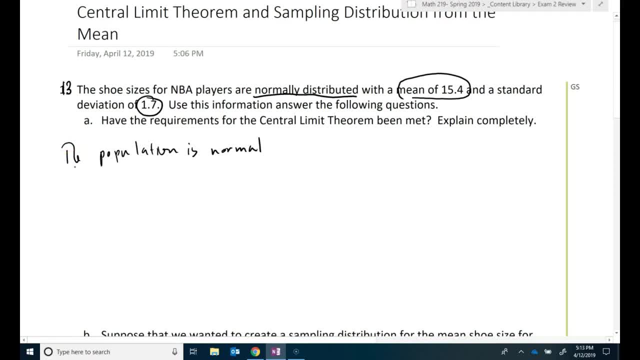 two possible requirements. There's not actually two requirements. We have to have one of two, Okay. One is we have to have either the population is normal- Okay, Or two we can have. the sample size is greater than or equal to 30.. 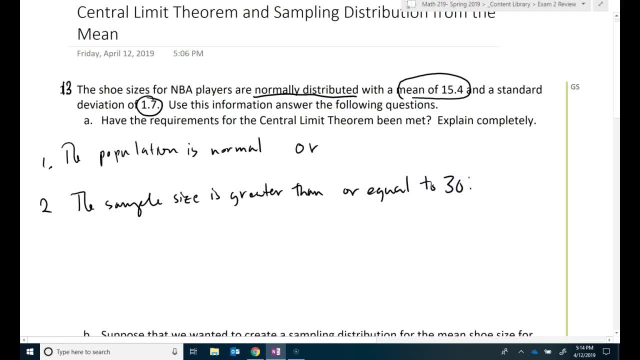 So what that means is this: If we know the population is normal, which is what, in this case, we do, the shoe size for NBA players is normally distributed. So all I have to say is: well, the shoe sizes for NBA players are normally distributed. 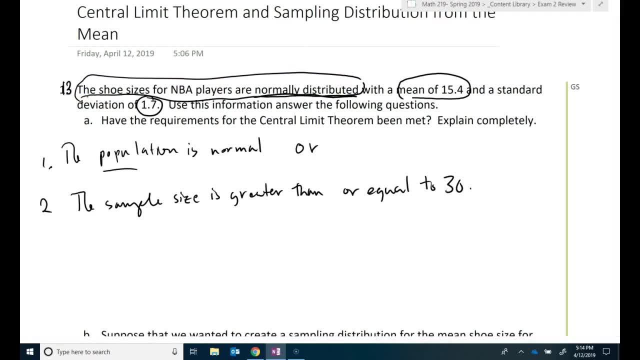 so the requirements for the central limit theorem have been met, okay, Or we know that the sample size n will be greater than 30, greater than or equal to 30. So if I know that that's the case, well then. 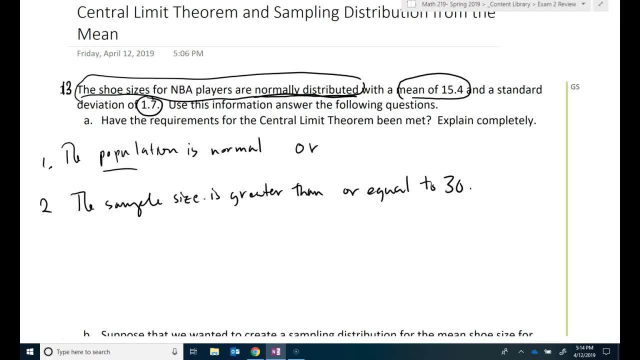 I also know that the central limit theorem conditions have been met. I only need one. only need one of these. Notice the or. So I only need one of them. okay, Consequently, if you know it's the population, it's normally distributed, you're done. 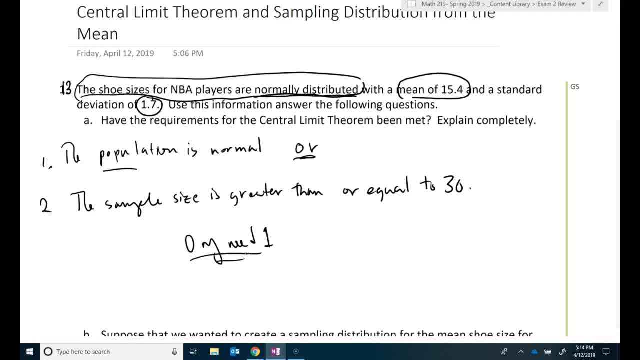 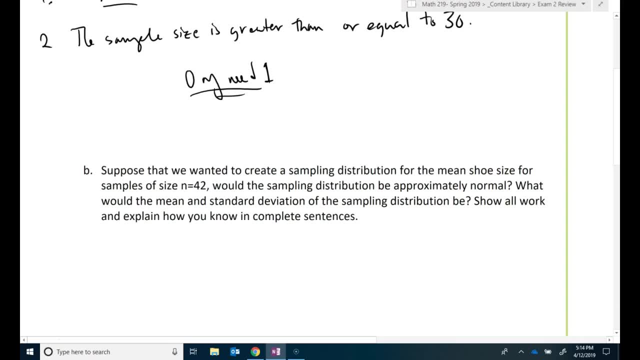 If you know, on the other hand, the sample size is greater than or equal to 30, you're done. Just mention one of them. okay, Now B suppose that we wanted to create a sampling distribution for the mean shoe size for samples of the size n equals 42.. 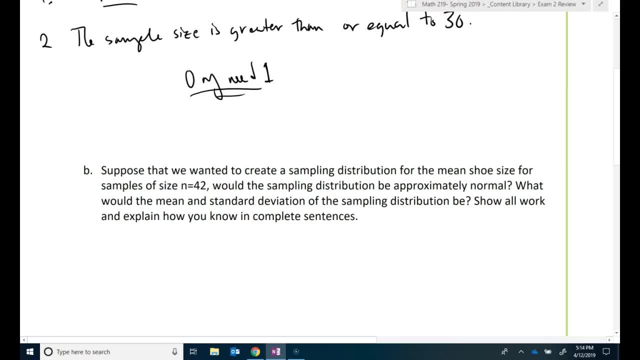 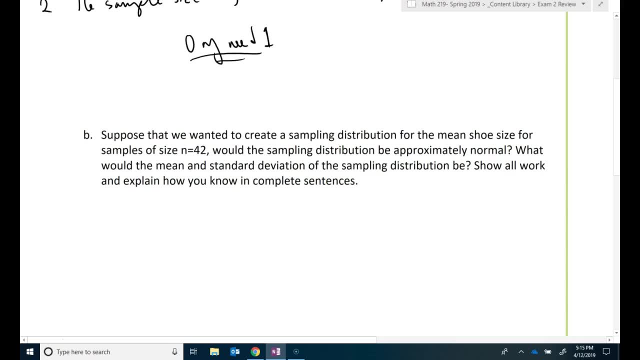 Would the sampling distribution be approximately normal? Okay, and then it asks us: would the mean and standard deviation of the sampling distribution be Okay? and then we want to show all of our work. Well, these are the requirements for the central limit theorem. 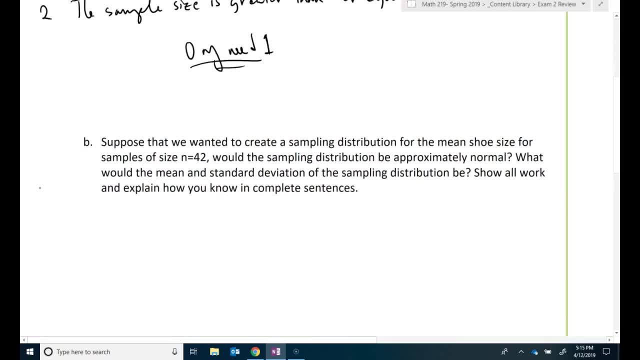 Okay, and then these are the results. We call them the results of the theorem. Okay, one is: the sampling distribution is approximately normal. The sampling distribution is approximately normal because we have met the requirements. Okay, Okay, The sampling distribution is approximately normal. 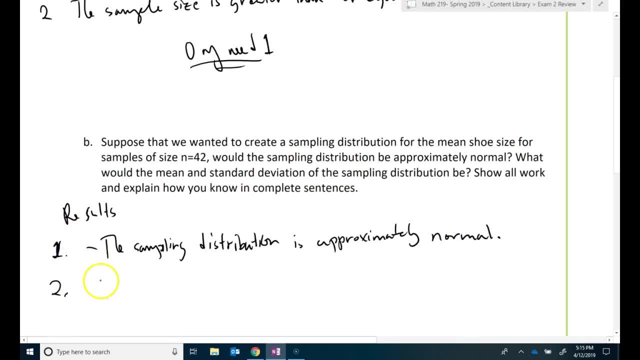 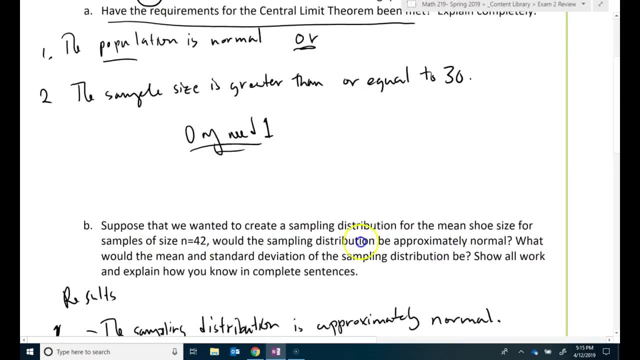 That's the first result. The second result is that mu of x bar, which is the mean for our sampling distribution, is equal to mu, which, in this case- oh well, that's not so bad, That's 15.4.. 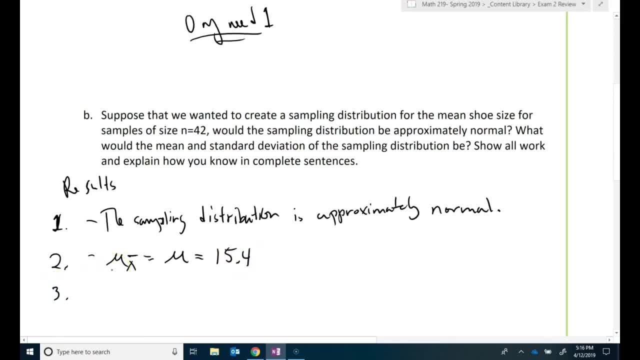 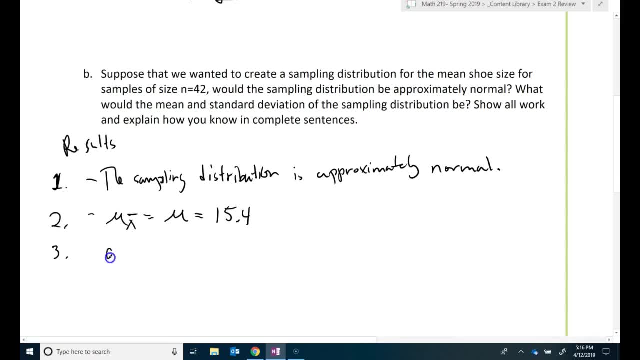 Okay, and then three. this one is the important one. that's actually really different. This changes everything about what you're doing for the sampling distributions. It's going to be: sigma of x bar is going to equal sigma over the square root of n. 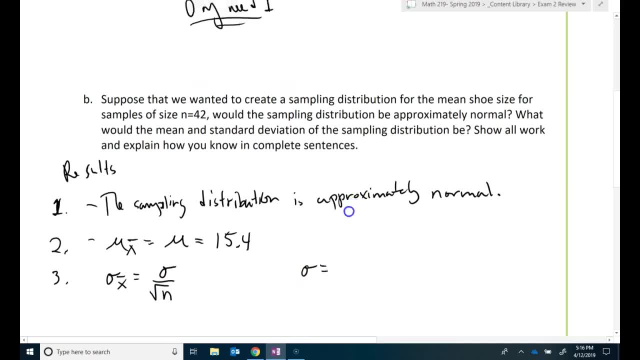 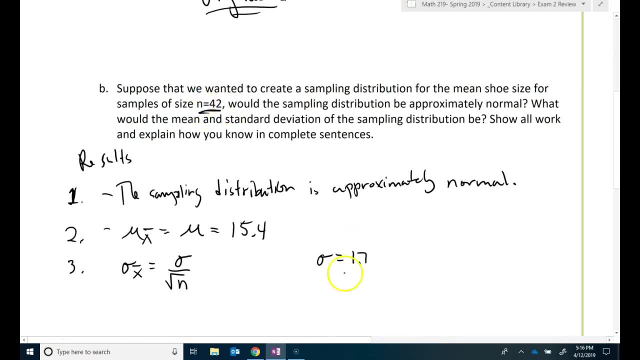 Okay. So sigma in this case is 1.7.. And notice n equals 42. So we get 1.7 divided by the square root of 42. Okay, And that's equal to 0.262.. Now something to notice here about that. 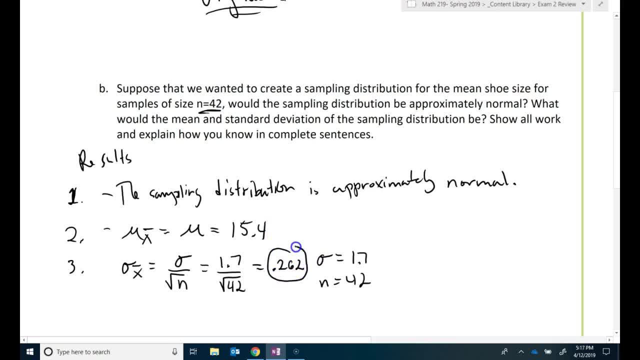 that's way smaller than 1.7.. So one of the things that happens when we generate a sampling distribution for the mean is we're actually asking about, like, the probability of getting average which is of a particular size. So, since we're looking for the probability of averages, 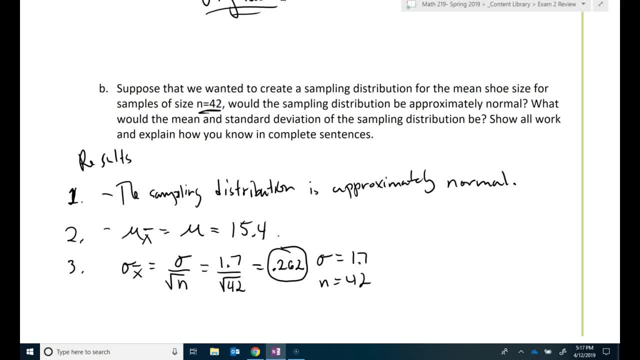 of a particular size, their standard deviation is a lot smaller because it's harder to get further away from the mean. I talked about that instead of the actual lesson as to, as we increase our sample size, our spread gets smaller and smaller because we're taking the square root. 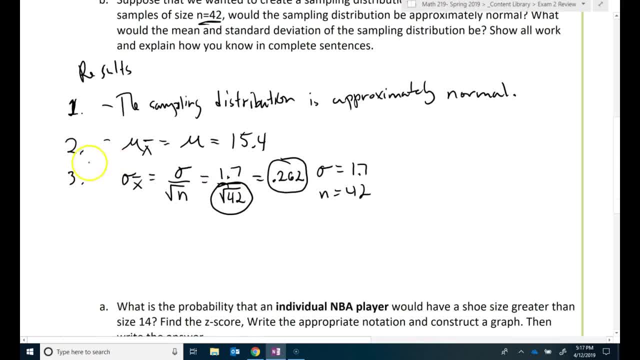 we're dividing by the square root of the sample size. So notice that These are the results. right? This is the big change. right here? That standard deviation ends up changing as a result of the central limit theorem. So anytime you're generating a sampling distribution, 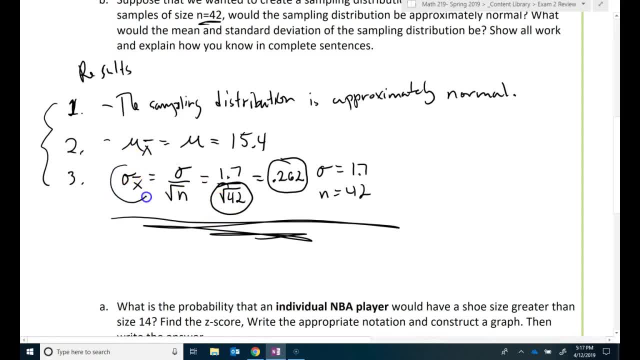 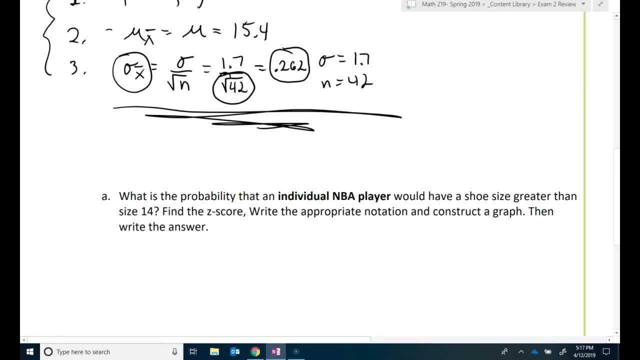 you need to use right this sigma of x-bar. Okay, Now what is the probability that an individual NBA player would have a shoe size greater than size 14?? Find the z-score, write an appropriate notation and construct a graph. 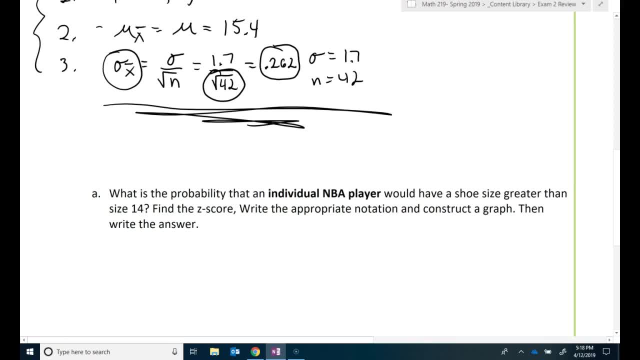 Then write the answer. One of the things that you want to notice is that this question is a lot like the one that we just did for the normal, The normal distribution. In fact, it's identical. Okay, And there's a reason why I highlighted. 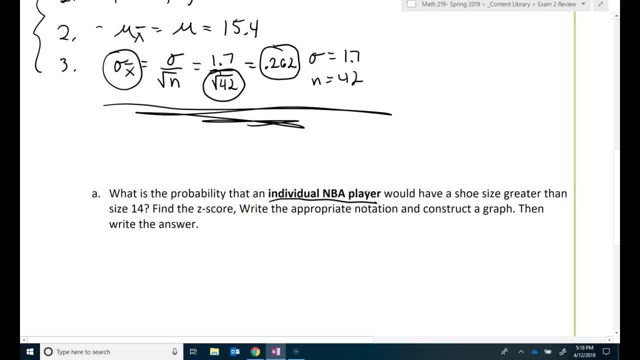 individual NBA player. It's because we are not going to use the central limit theorem or the sampling distribution for this question. Sampling distributions are for samples and for averages. Okay, This is an individual and it's out of a population, So we're going to have 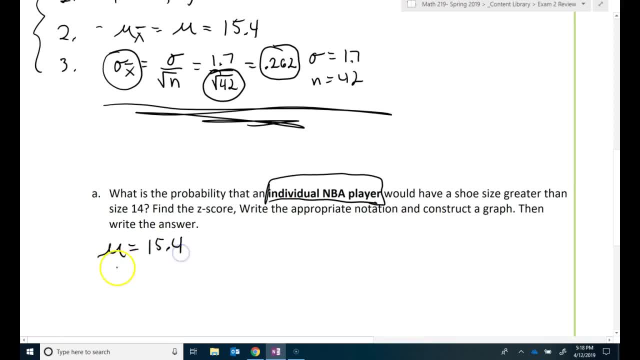 I'll write my mu mu equals 15.4.. And remember when I said that big difference- it's a sigma here- now is 1.7.. Right, Because we're looking for the individual NBA player. Okay, So, and then our x here is going to be equal to 14.. 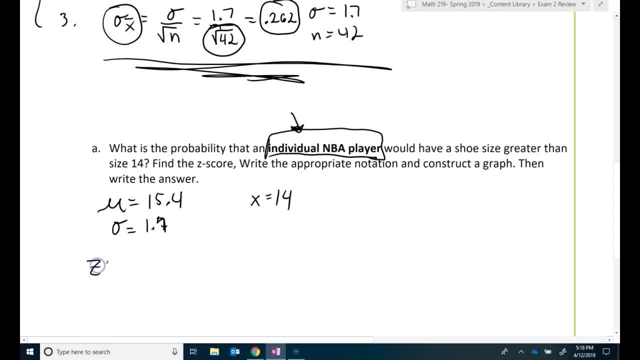 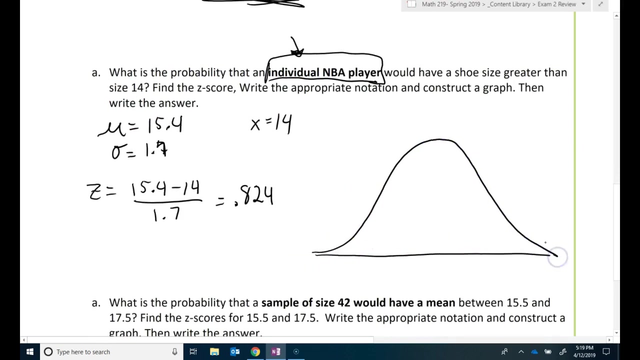 So z our z-score will equal 15.4 minus 14 divided by 1.7, which will equal 0.824.. Okay, Now I'm going to draw my distribution. Oh, by the way, I should write my notation, huh. 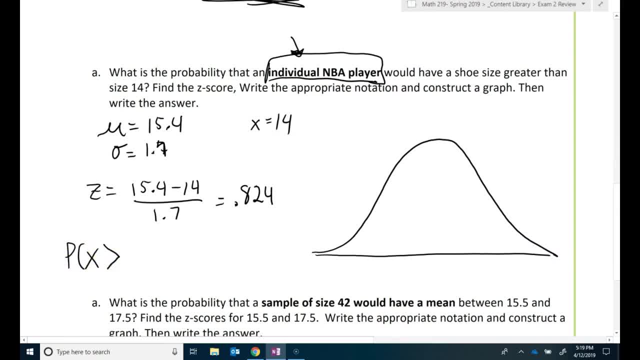 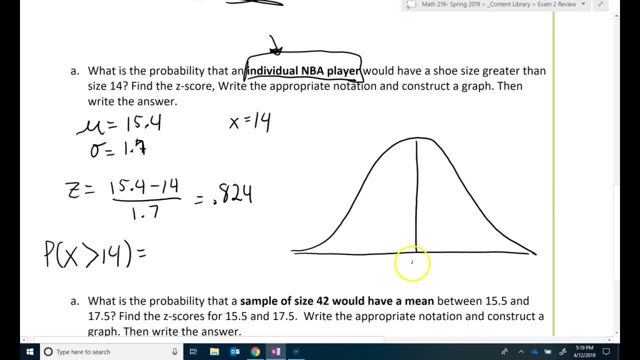 Probability that x will be greater than 14.. Really important too, because, notice, it's a greater than sign. So I have here's 15.4.. 0.824.. 0.824.. That's right about here. It's a little bit less than one standard deviation. 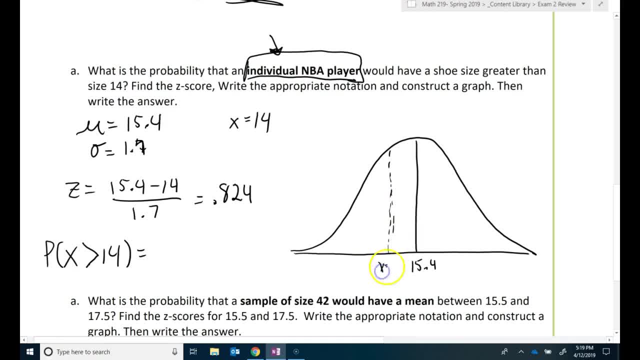 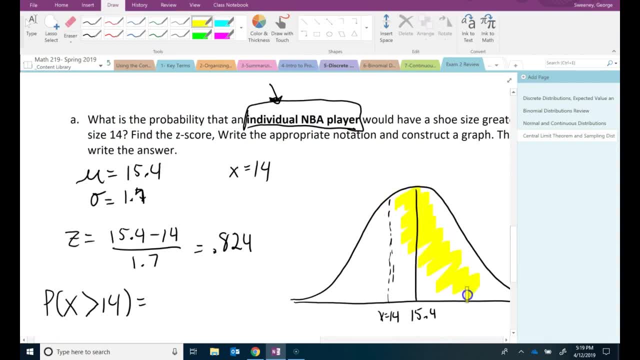 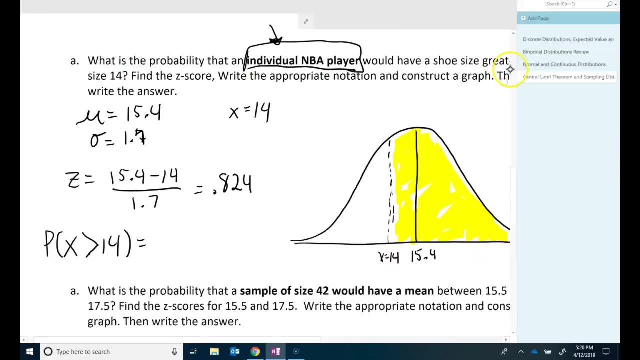 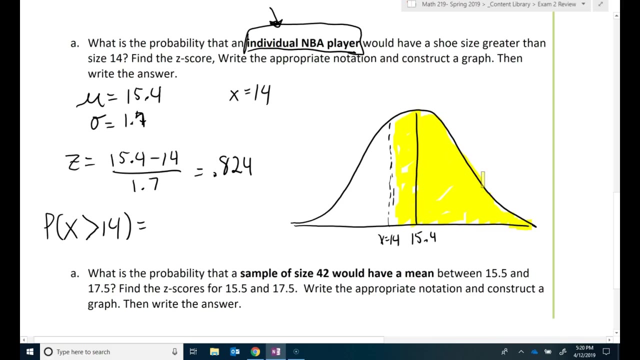 away from the mean. So there's 14.. x equals 14. And then here's the value of x, And we just go ahead and we'll shade it out. There it is Done, Ta-da, Okay. Now I'm going to go in. 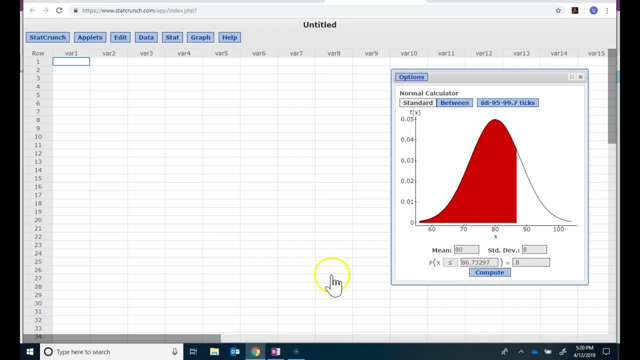 I'm going to go to StatCrunch. I'm going to put in my mean and my standard deviation. So 15.4 is my mean, My standard deviation is 1.7. And I want to know the probability that x is. 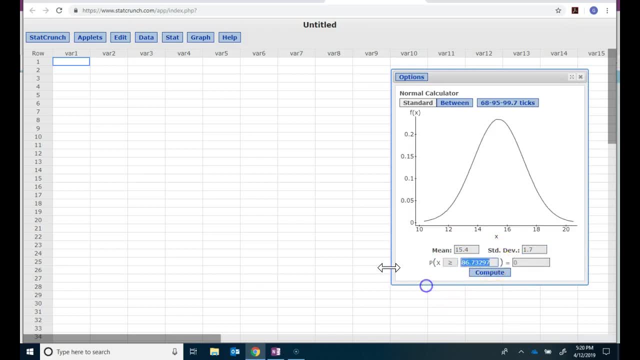 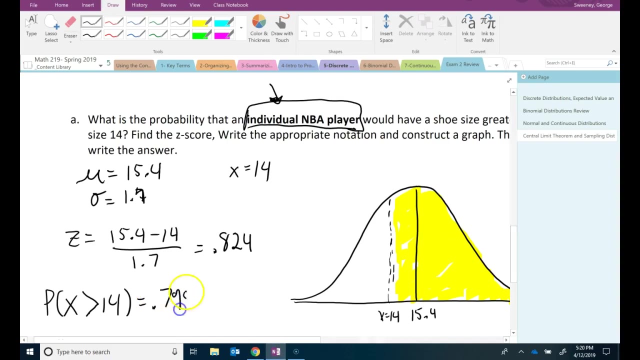 in fact greater than or equal to 14.. I compute And there it is 0.795.. That makes sense to me. Looks about right too right. Okay, That looks it's quite a bit more than 50%. 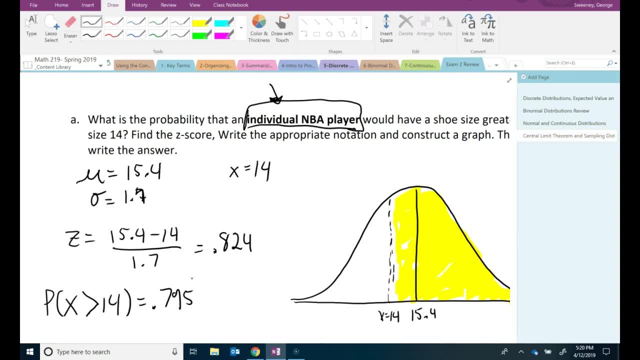 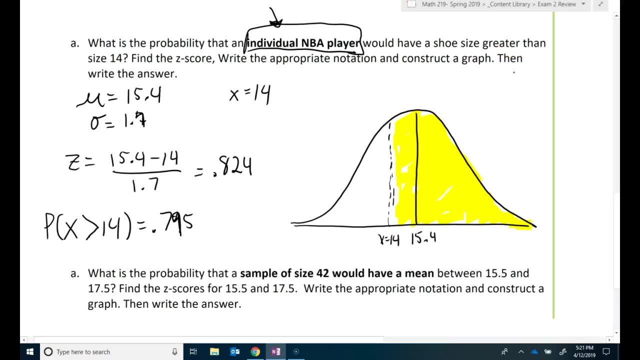 Right, It's almost 80% of the entire distribution. Okay, All right, Cool, Now let's take a look at. this actually ends up being d. This is d. What is the probability that a sample of size 42? 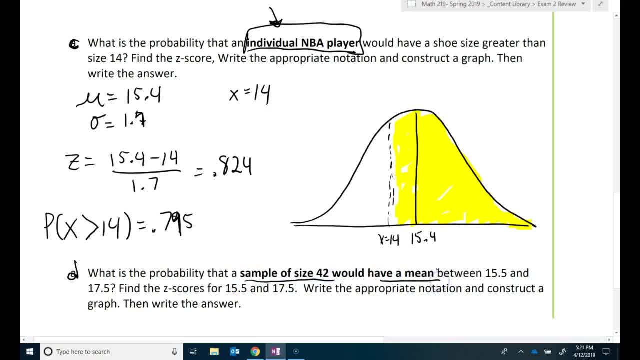 would have a a mean of between 15.5 and 17.5? All right, Well, first one thing that I first want you to notice. it's a sample of size 42, and we're looking for the probability of a mean existing. 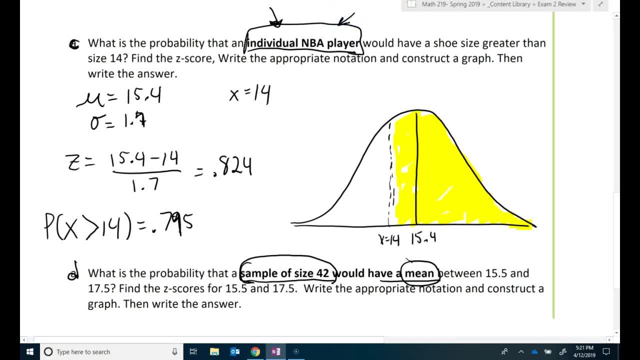 versus individual NBA player. You guys get that. So now what we're looking at is: if I pick 42 players at random, what's the probability that one out of those 42 players or, excuse me, what is the probability that the average foot size 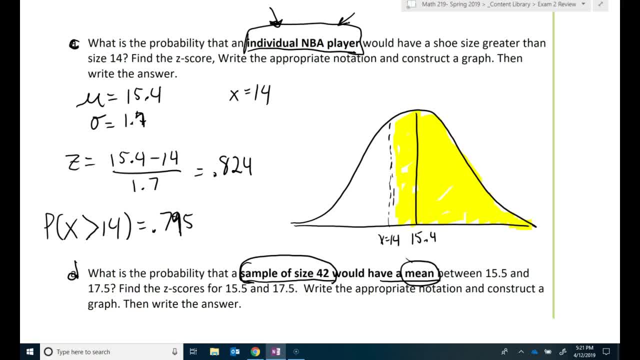 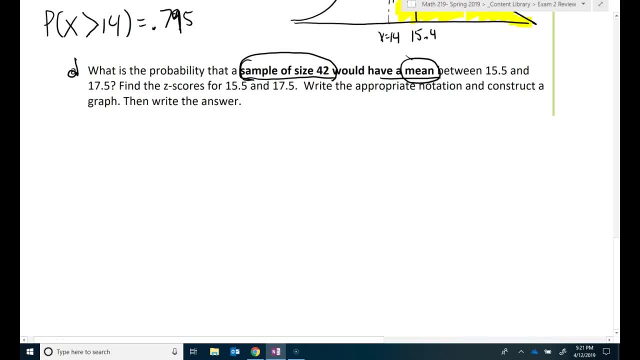 for those 42 players is going to be between 15.5 and 17.5? Okay, Now, now that I've identified that I'm looking at sampling distribution for the mean right- Okay, Sample, mean right. 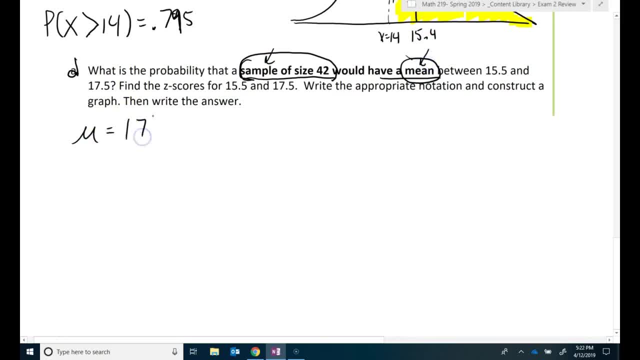 I now have mu is going to be 17, or, excuse me, it's 15.4,, just like it was before. right, Because mu of x bar equals mu of x equals mu. Then sigma of x bar, right. 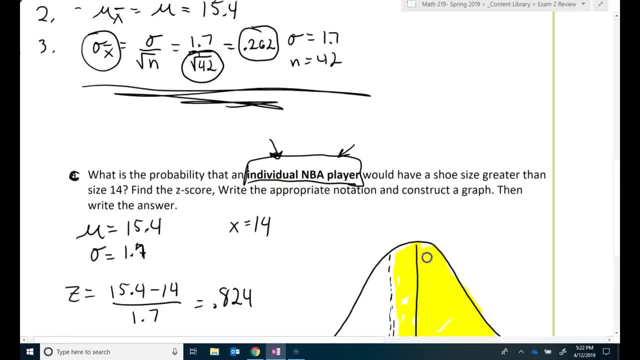 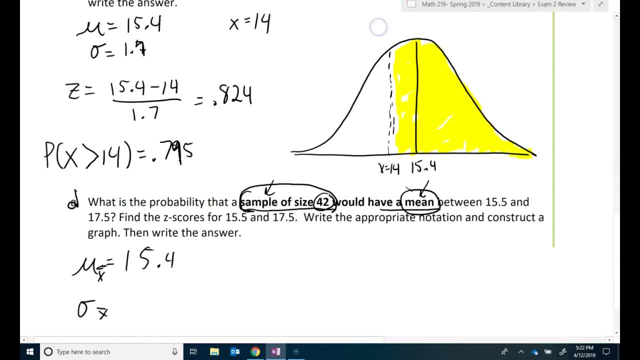 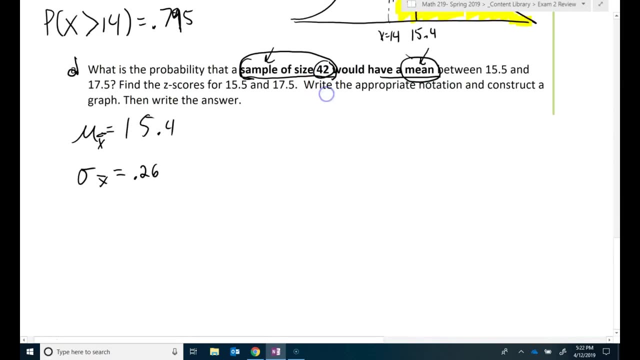 We found it for size 42 already. All right, sigma of x bar is going to be this value here, right, The 1.7 over root 42.. So that's 0.262, 262,, that's 262,, yeah, 262.. 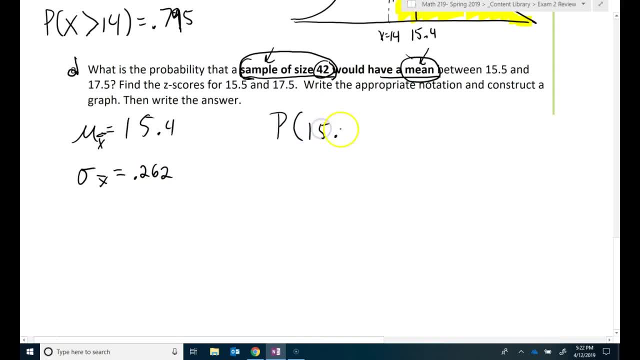 We're looking for the probability that x is between 15.5 and 17.5, right, Okay, And so now I need to find my z-scores. So the z-score for 15.5 is going to be 15.5 minus 15.4. 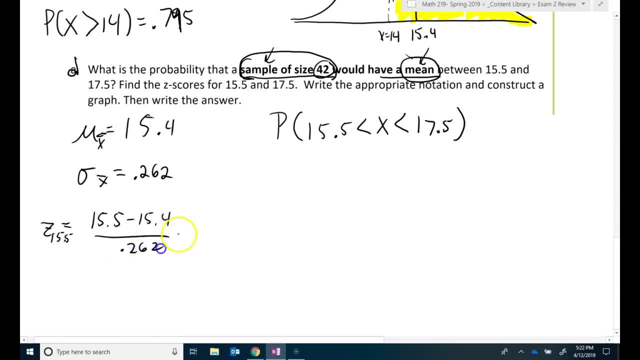 divided by 0.262, right, That's going to be very different than if we utilized 1.7.. I promise you that 0.382.. Then we'll take the z-score for 17.5.. Now you're thinking to yourself. you know what? 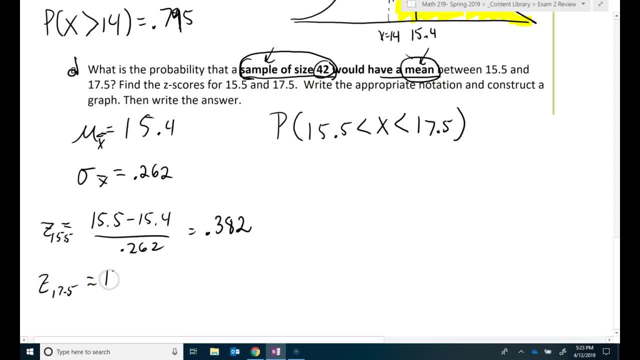 It's only like 2.1, so it shouldn't be that big, But we're going to go through it and divide it through by 0.262.. Hmm, Wow, That's going to end up being really far away from 0.262.. 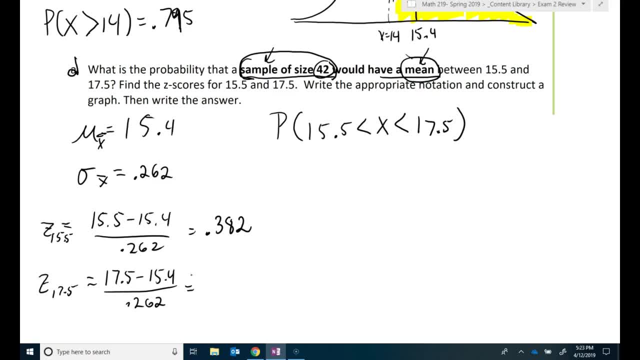 So we're going to go through it and divide it through by 0.262.. Hmm, That's going to equal 8.015.. So it's 8.015 standard deviations away from the mean. It's like a ridiculously far distance away from the mean. 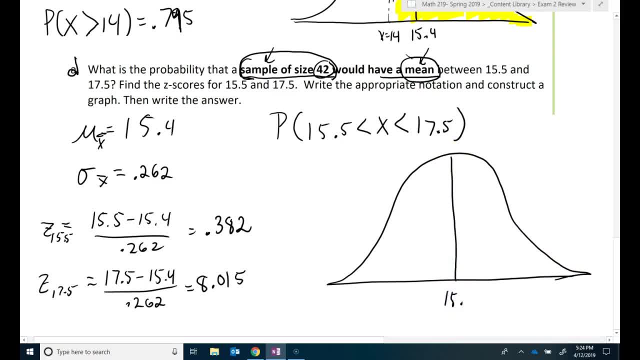 So we've got here. here's 15.4.. We start out. we're going to start out about halfway, like a little less than half a standard deviation away. So there's 15.5.. Notice that, even though it's only 0.1,. 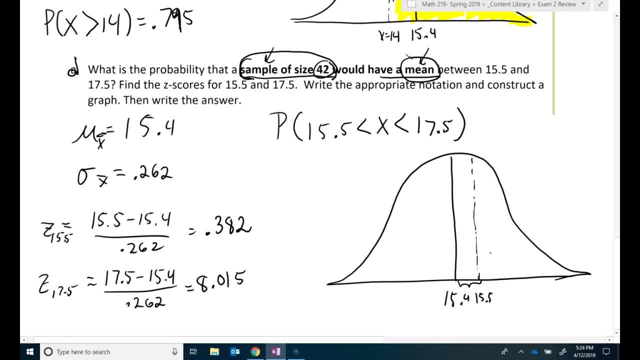 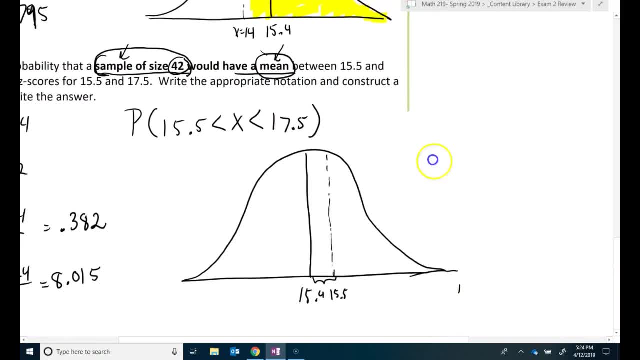 it's pretty far away. Okay, So it's 0.382 standard deviations away, And then 17.5 is is. I mean, like you know, it's out here, Here's 17.5.. It's so far out. 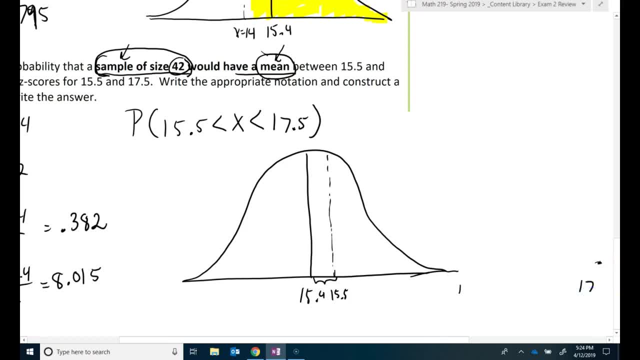 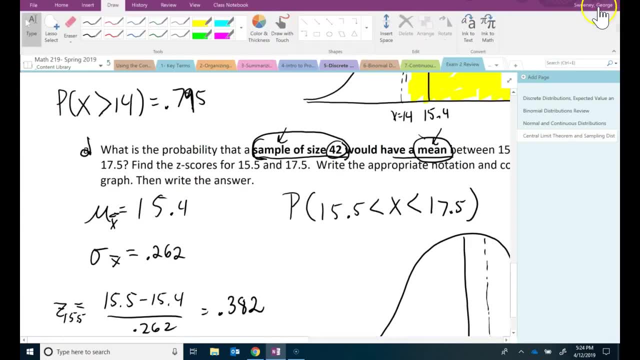 It's not even like on the range when we use the imperialism. So it's way out there. So we're not even- I mean like we barely even have to worry about it. So let's just go in here. 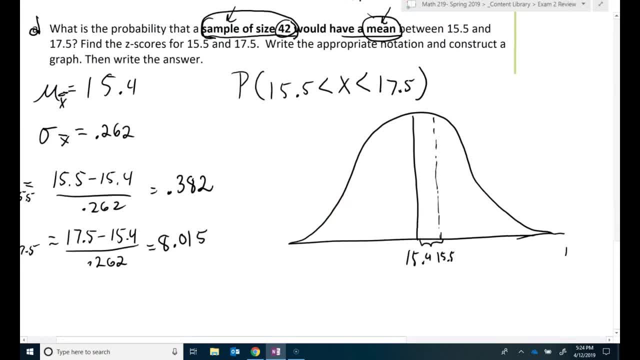 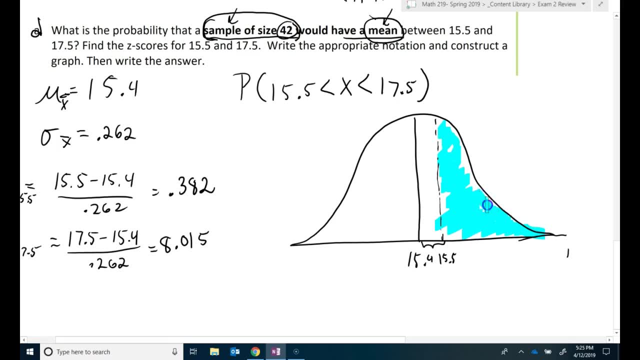 We'll now draw a picture, Or but. but we're good. So anytime you have a standard deviation like a z-square that's bigger than- oh, I don't know- four, or really three, it ends up. 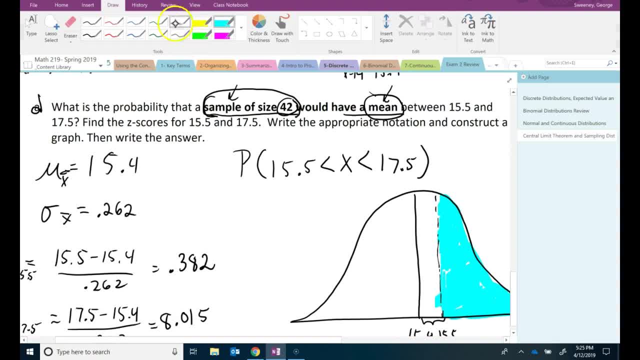 it's. it's so far away that it barely adds anything to the overall area. Right, It's like it's basically the equivalent of if we said, OK, go all the way out to the end, OK, So there's that. 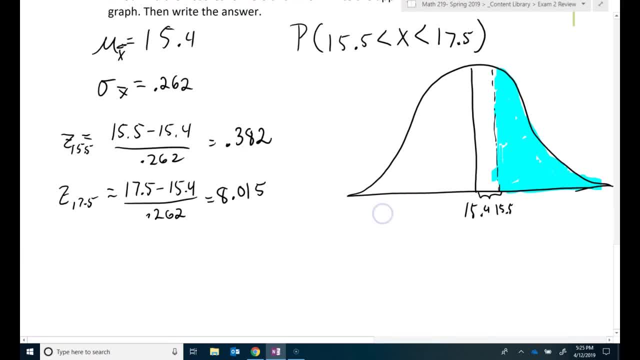 There's our picture And now we'll go in take 15.4.. Now notice something: If I had kept it at 1.7, watch this. OK, Take 15.5 to 17.5.. 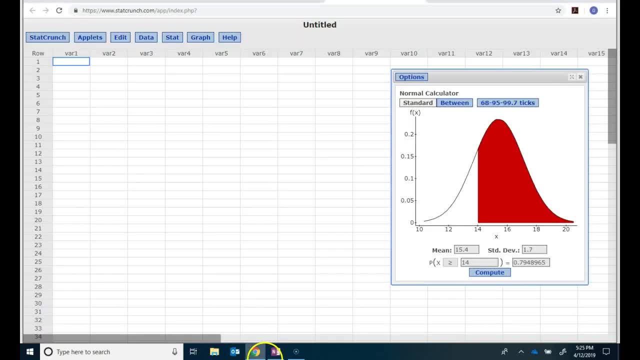 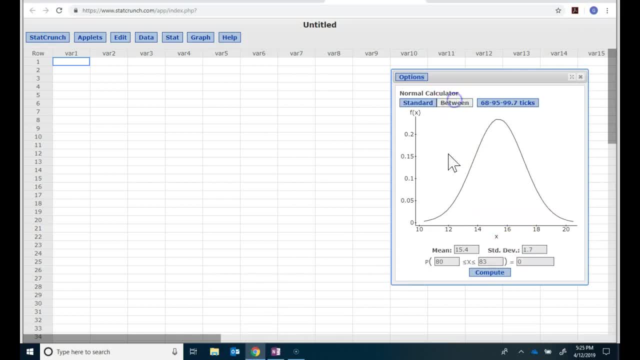 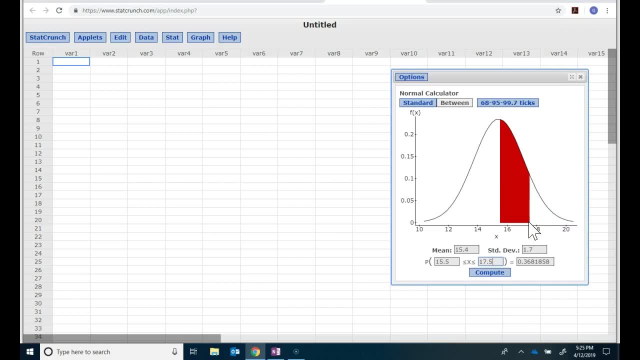 deviations away from the mean. Okay, It's like one and a half, So, wow, that's going to be really far off. But when I go in, oh and sorry, let me just- actually it's going to be 0.368, right. 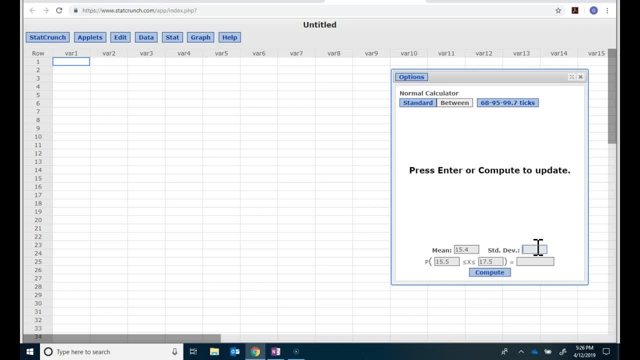 That's the probability there. Let's just do a comparison now to when we have 0.262 as my probability, as my standard deviation. Oh wow. Now what you're looking at is it's way farther over and we're actually bubbling in the entirety of the distribution like the end of the. 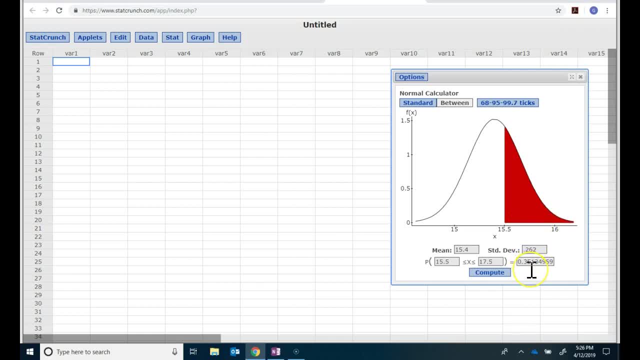 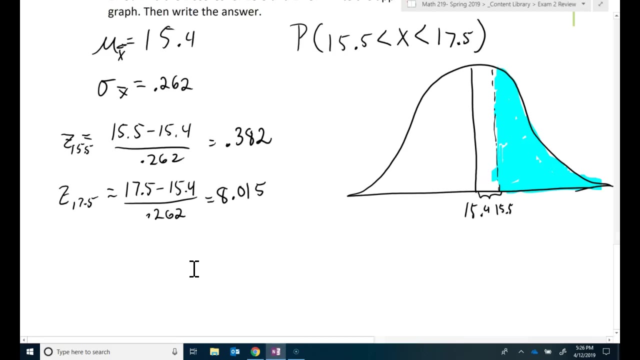 distribution, the whole tail of that distribution, And our probability now is 0.351, mostly because we've actually dropped off a big chunk of the middle part. So 0.351.. Okay, Get how different those pictures are. All right, 0.351.. 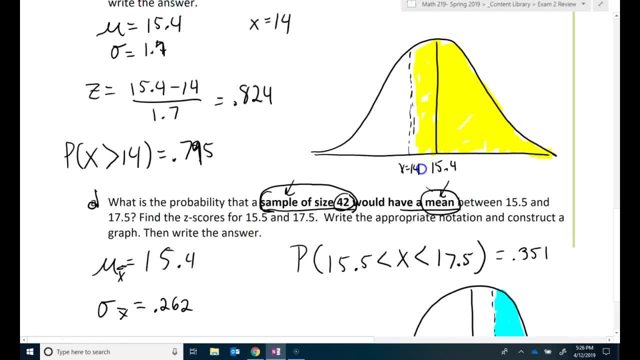 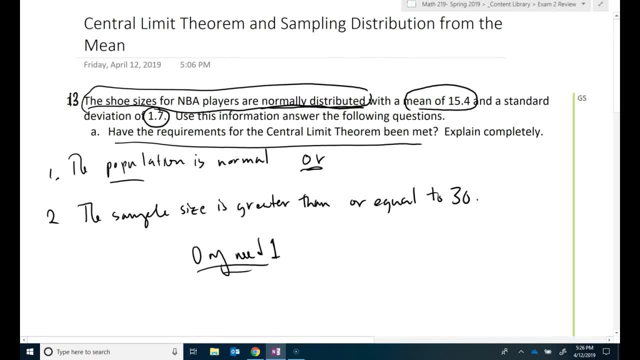 Okay, Cool, All right. So what do you need to know, or what are some of the most important things that you need to know to work with the central limit theorem and sampling distributions for the mean? Well, the first is is that we're going to utilize the central limit theorem.